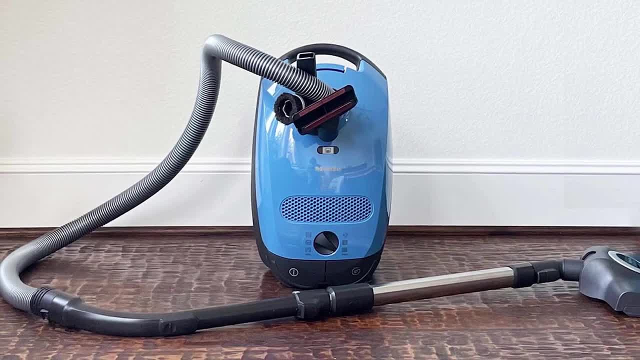 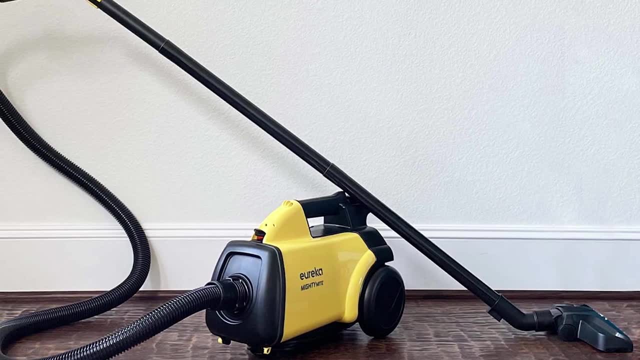 quieter than that average around 60-65 decibels. Contrast that with the quietest upright vacuums, which clock in at about 70 decibels. While a few dBs might not seem like much, the decibel scale is logarithmic. Simply put, 73 dB is twice as loud as 70 dB. 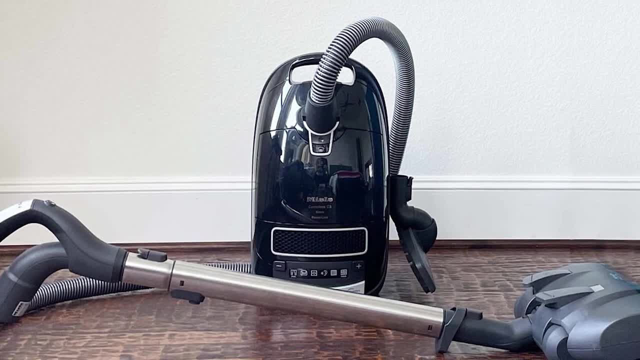 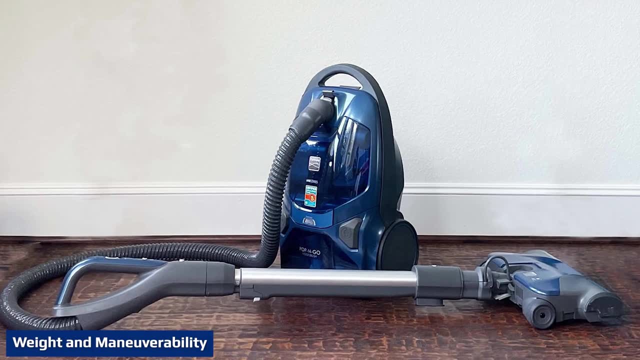 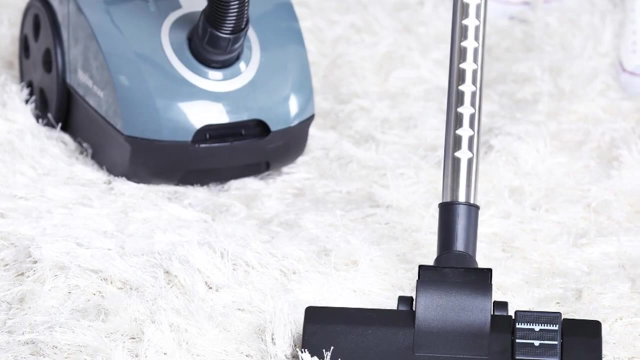 and half as loud as 76 dB. If you or anyone in your household is especially sensitive to noise, canister vacuums are the clear choice. In general, canister vacuums tend to be slightly lighter than upright models. While the difference might only be a few pounds, the design of canister vacuums makes them feel. 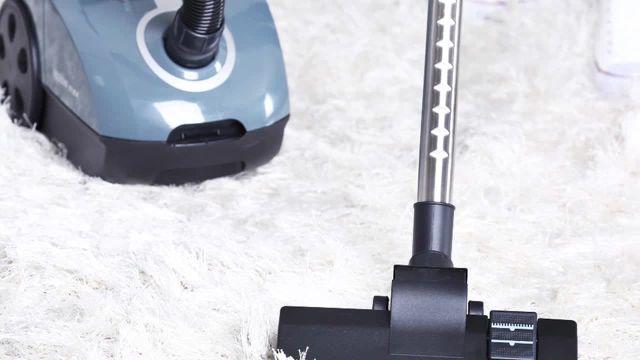 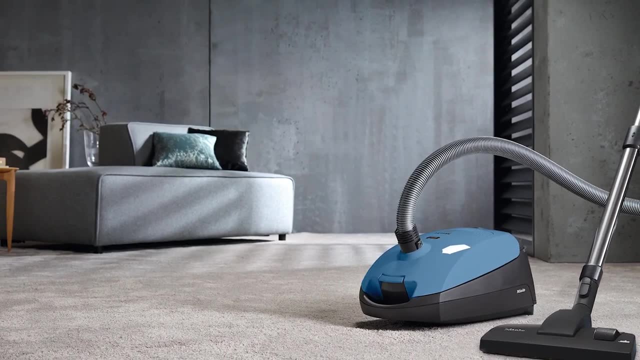 much lighter Rather than pushing and pulling the full device across the floor. the majority of a canister vacuum sits stationary while you use the lightweight one and the attached head to clean. Canister vacuums are not as loud as 70-60 dB. 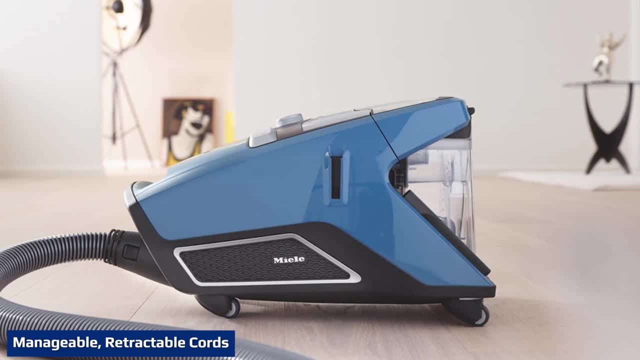 Almost all canister vacuums are loud. Canister vacuums are loud. Canister vacuums are loud. Canister vacuums offer retractable cords which hide inside the canister when not in use. This feature provides the vacuum with a cleaner appearance and reduces the chances of tripping over the cord. If you've 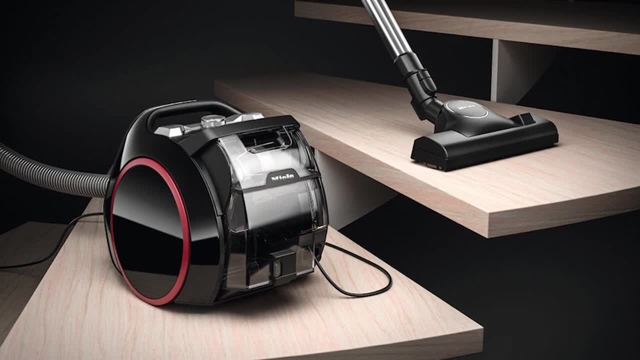 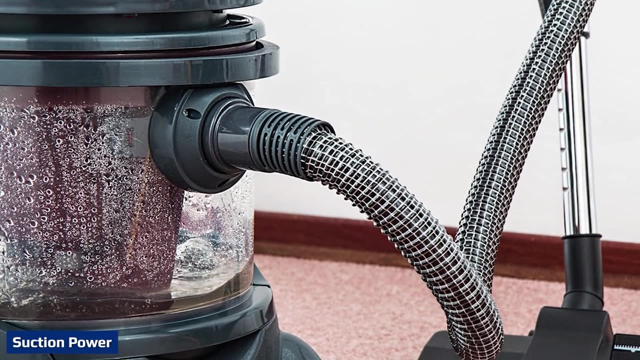 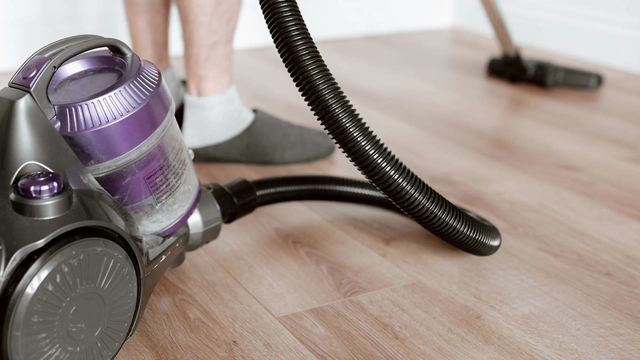 ever done this, you know how annoying and potentially painful it can be. Canister vacuums generally have more suction power than upright models. This power makes them particularly well-suited for cleaning bare floors, And, while they are also efficient at cleaning carpets, upright vacuums tend to be more effective carpet cleaners. 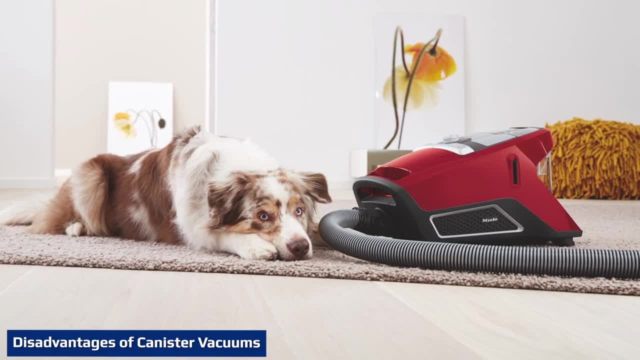 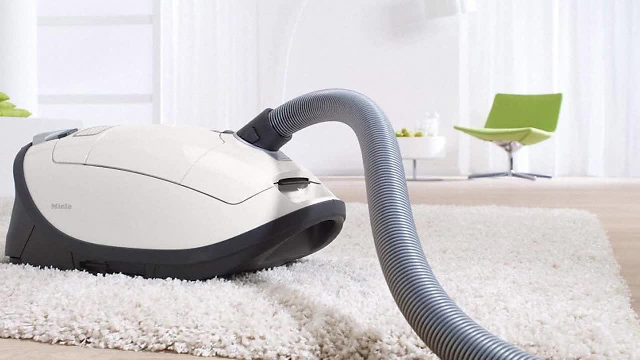 Not easy to store. Although the wand and head of a canister vacuum is more maneuverable than upright vacuums, the canister itself can be cumbersome. Rather than having a single unit to move around, you have two pieces to worry about For small spaces: the hose connecting 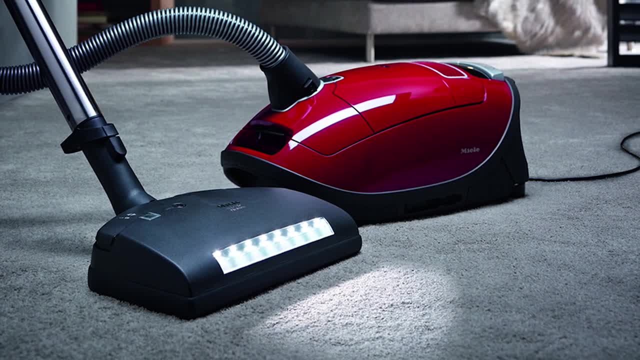 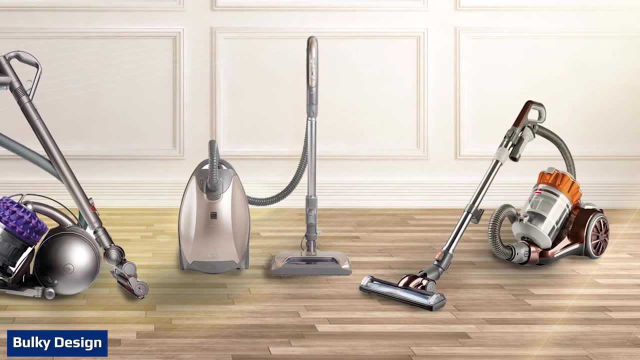 the canister to the wand is usually long enough that you won't have to move the canister much. Because of their disjointed design, canister vacuums are not as easy to store. Upright models typically balance on their head, making them easy to tuck away in the canister. 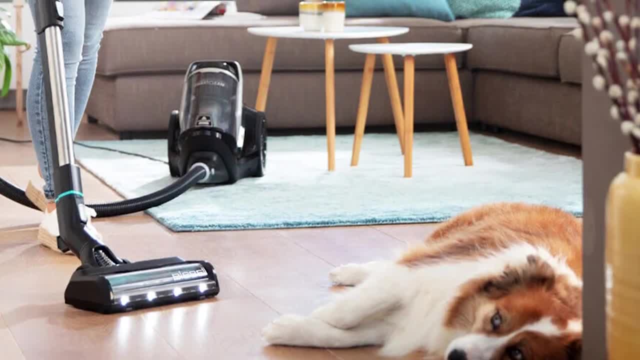 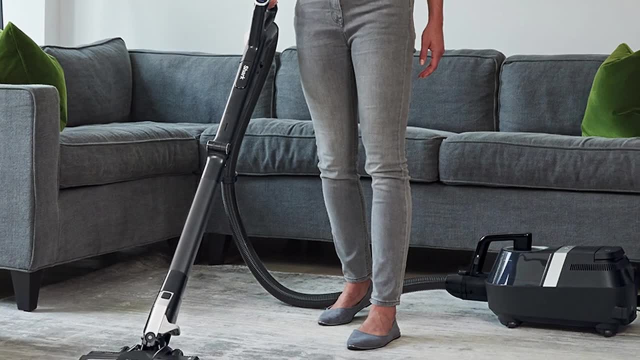 While the canister portion of a canister vacuum is stable enough, the hose, wand and head generally can't stand on their own accord. They should still fit in just about any closet. Just know that they'll take up a bit more space, and the wand's heads have a habit of. 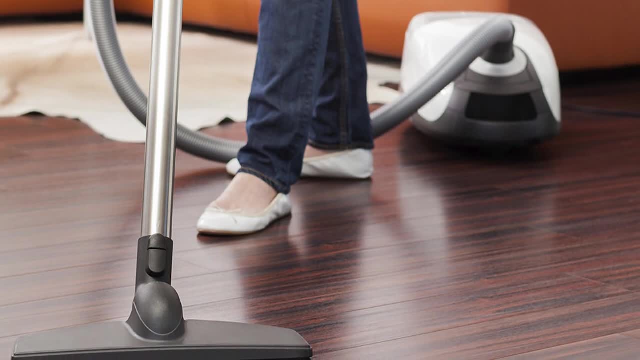 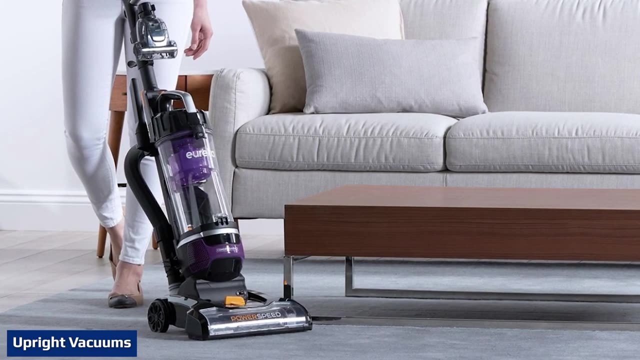 falling over if they aren't carefully balanced. Advantages of upright vacuums: Easy to use. The one-piece design of upright vacuums makes them easier to move from room to room Rather than bending down to deal with the canister. the handle on upright vacuums lets you. push, pull and slide the canister to the side of the canister. This allows you to move the canister as far as you can. You don't have to push the canister to the side of the canister. You can also. 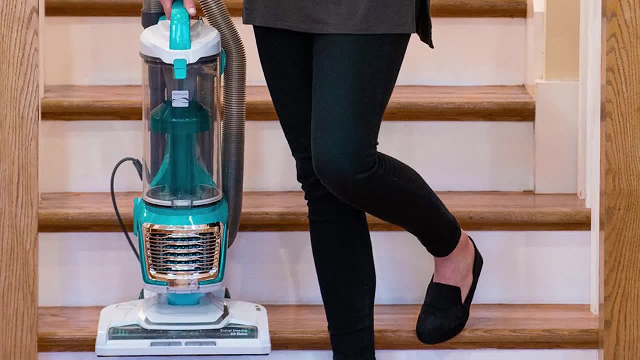 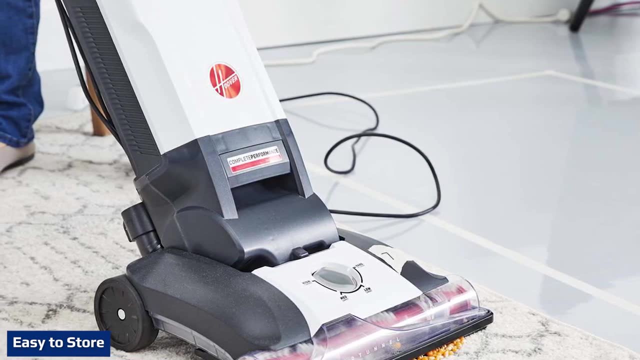 pull or carry the whole device with a single hand. Upright vacuums can easily stand up on their own inside a closet or anywhere else you have a place for them. Some models even offer customized wall mounts that help free up floor space in your mudroom, garage or wherever your vacuum lies. 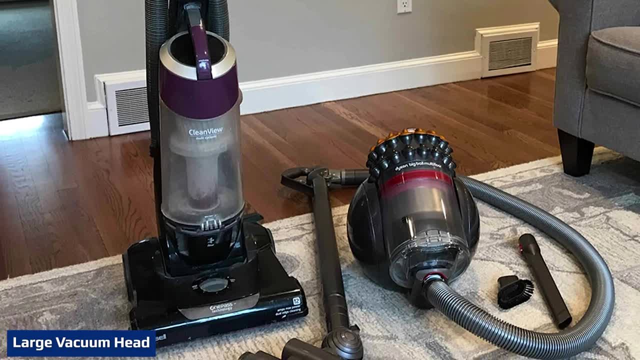 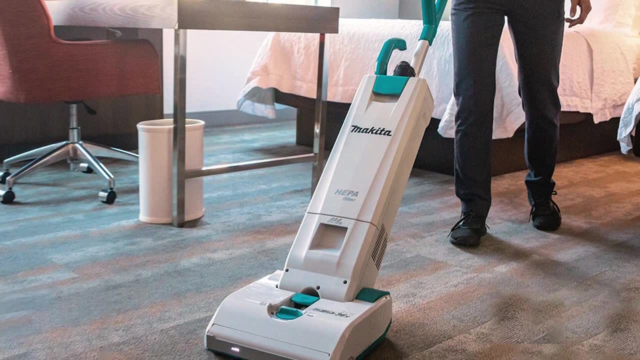 The large head that allows upright vacuums to balance on their own also comes in handy when vacuuming large areas. Its wide footprint makes it easy to quickly clean even the largest rooms. Most upright vacuum models are bagless, built instead with plastic receptacles that can snap. 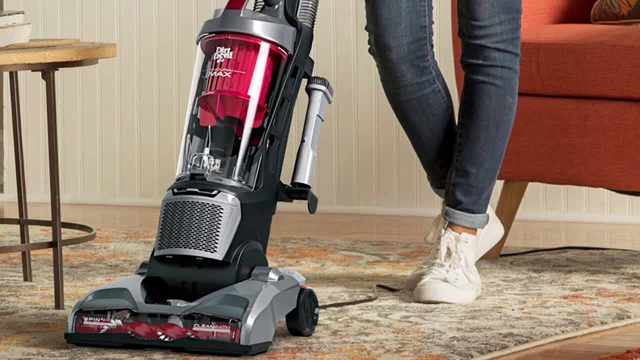 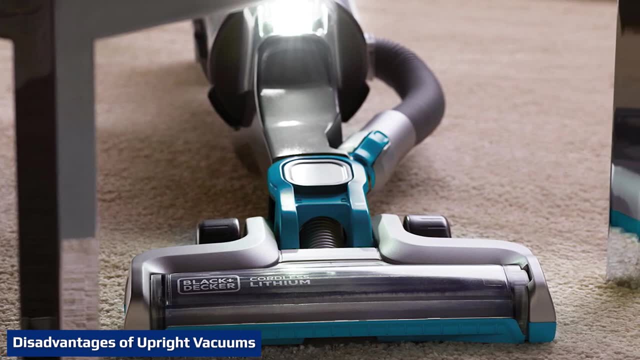 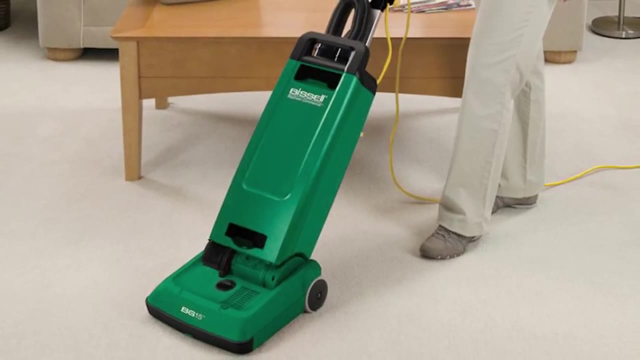 in and out of place. This makes them significantly easier to clean once you finish collecting all the dirt and debris. Nice level, As discussed above, upright vacuums are almost always louder than canister vacuums. You can still find a quiet upright vacuum rated around 70 decibels, but in general, 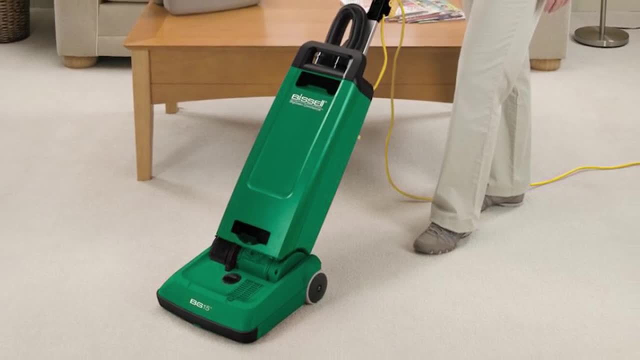 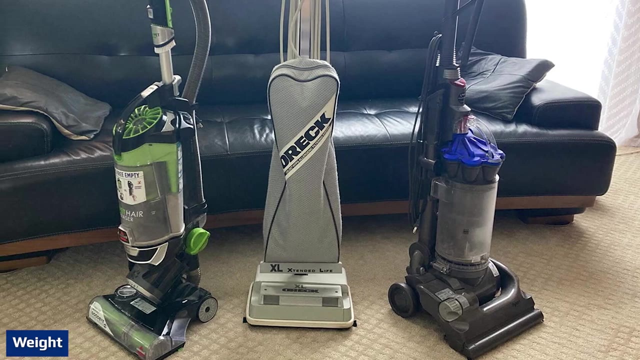 their unibody design makes it hard to muffle the sound from the motor. Upright vacuums can weigh 20 pounds or more. That might not sound like too heavy, given that you don't have to fully lift them off the ground very often, but their weight becomes more and more noticeable the longer you 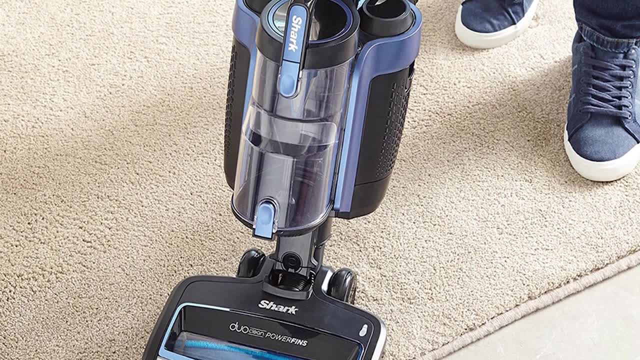 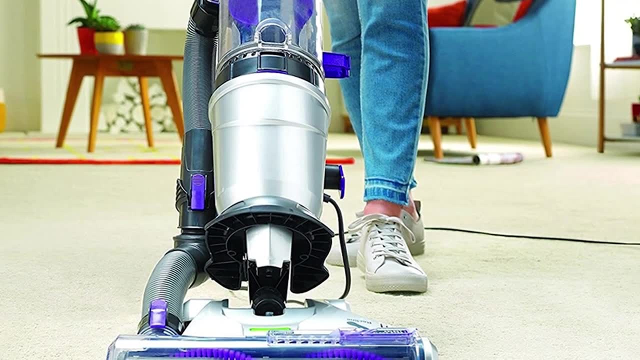 vacuum. However, there are some lightweight upright models weighing just 10 pounds. If weight is a big concern, a cordless stick vacuum could be a better choice than either a canister or upright model. Unlike canister vacuums, upright vacuums can't reach all those. 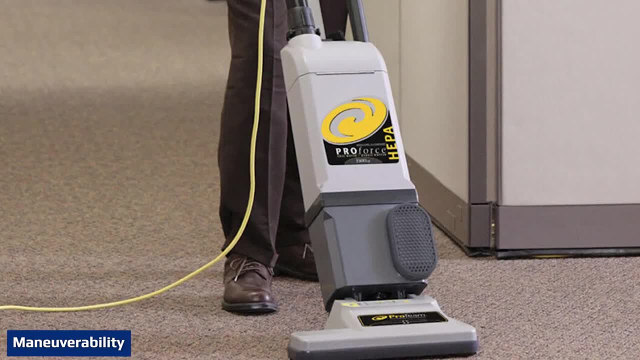 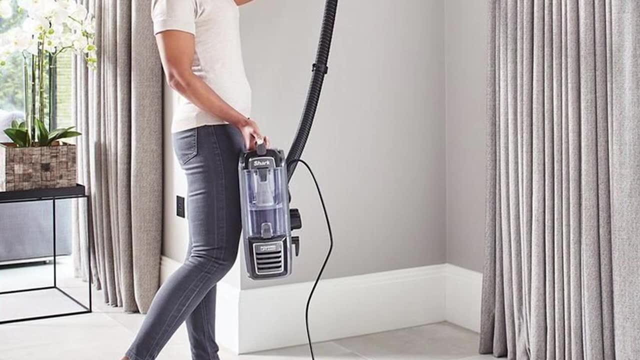 corners and crevices. Sure, you can add attachments, but it can still be awkward to reach behind and run furniture. Stairs are also a pain to vacuum with an upright. They require you to lift their heavy frame from step to step, Plus, their wide head might be bigger than the steps themselves.